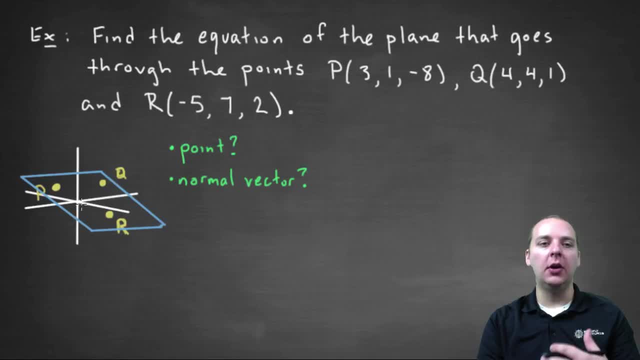 would look like. Let's think back over the last few videos here. What do we need to identify or write the equation of a plane? Well, I think we need two things. We need any point that is in that plane And we need the normal vector to the plane. These are the two things. 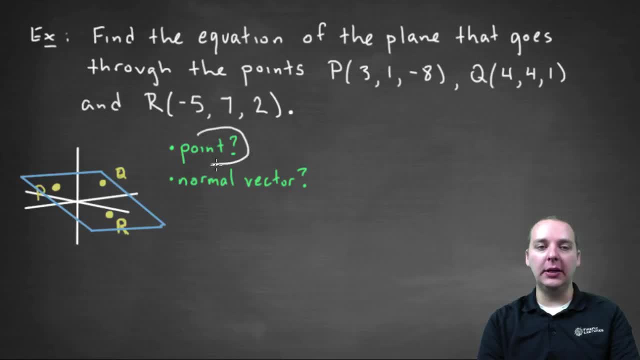 we need Now. we actually have an overabundance of points. We've got all the points we can handle. We've got tons of points that are in the plane. P, Q or R would suffice. But what I don't have is a vector that is normal, which means orthogonal to the plane. That 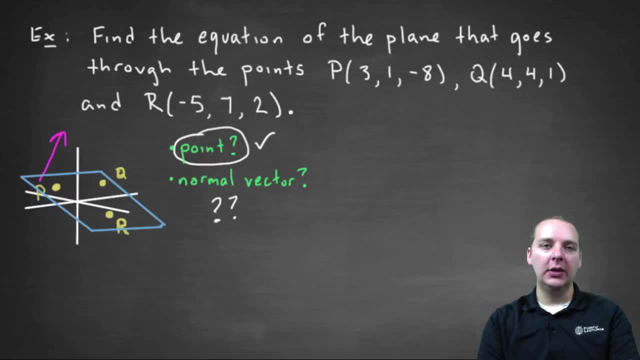 means it meets it at a right, at a right angle. So that's really going to be the, that's going to be the biggest issue we're going to have to deal with. So think about it for a minute. Can you think of a way and pause the video if you need to? Can you think of a way of? 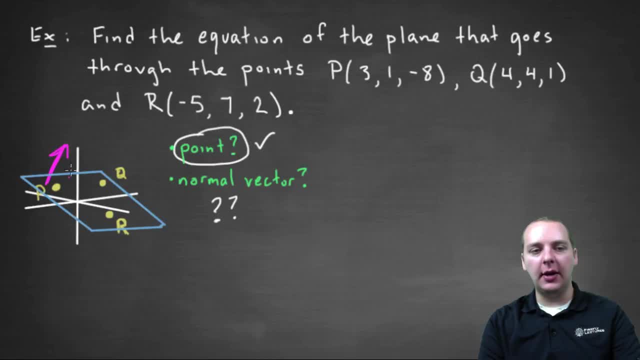 finding a vector that would come down and meet this plane at a 90 degree angle with the points P, Q and R, provided. Okay, hopefully, here's, here's what you came up with. This is here's a pretty clever idea, Um, and, and this is really once you, once you get. 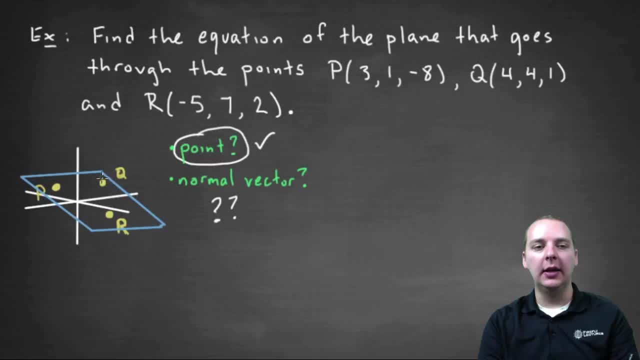 this part down, The rest of the problem goes pretty smoothly. Um, we can create vectors between these three points. We can, you know, for example, make a vector from P to Q, And we can make a vector from P to R. let's say So, these two vectors are in the plane. Now, do you remember something? 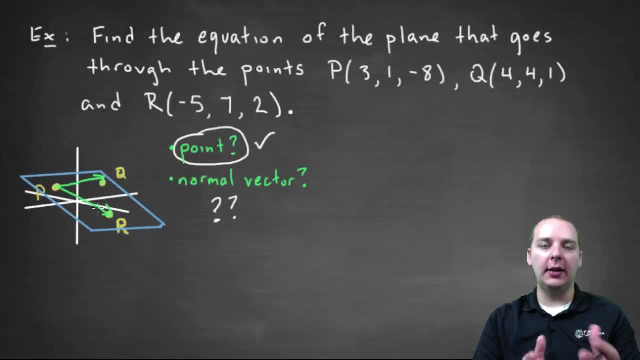 we've done fairly recently that can create, that can take two vectors and somehow use these two vectors to create a new vector that's or something that's going to be in the plane. It's going to be orthogonal to both of those guys at the same time. Hopefully you're thinking. 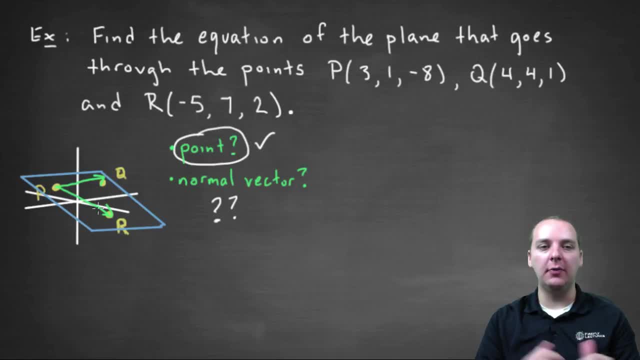 of a cross product. If you don't remember it, go back and watch our cross product videos. But if you take the cross product of P and P Q and P R, you'll get a vector like this pink one here that is orthogonal to both of these guys at the same time. So that's. 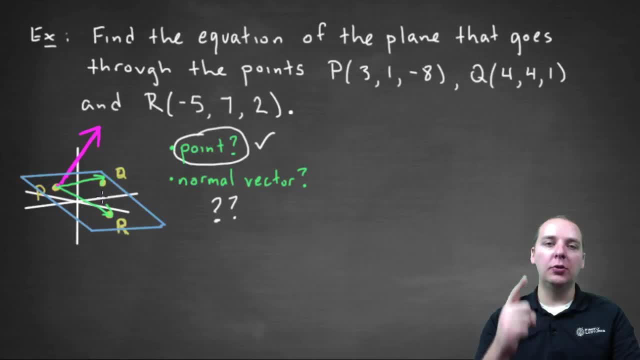 gonna be the process. We're gonna create a vector P- Q, We're gonna create a vector P- Q and R. Then we're gonna take their cross product. That new vector, the cross product vector, is gonna serve as our normal vector to the plane, Because if it's orthogonal to 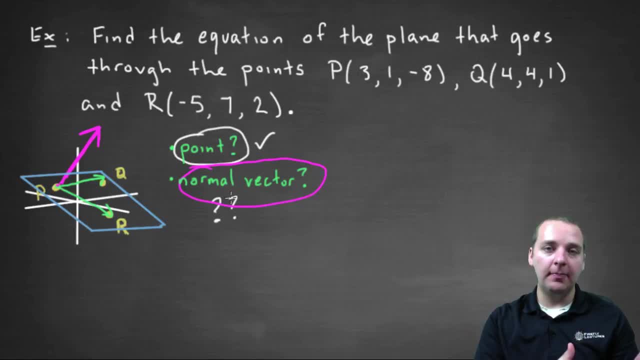 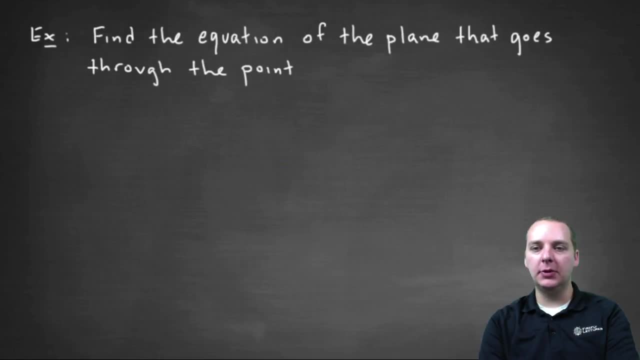 both of those vectors and those vectors are in the plane, then it would be orthogonal to our plane as well, of course. Alright, so let me, let me clear out some of this stuff, just so we have some, some room to write. Um, here I've copied P, Q and R, just to 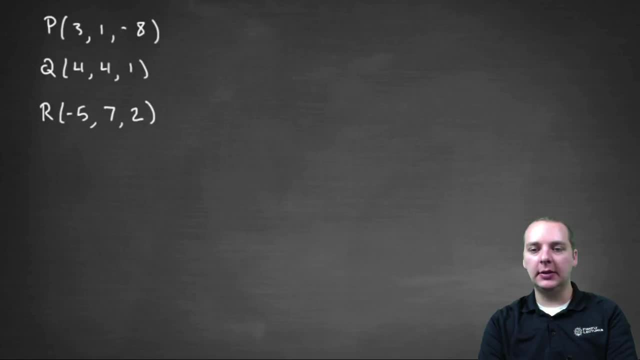 give us some, some space to write some stuff down And let's, let's go forward. Okay, so first off, we'll create P Q and then we'll create P R, P Q and P R To. 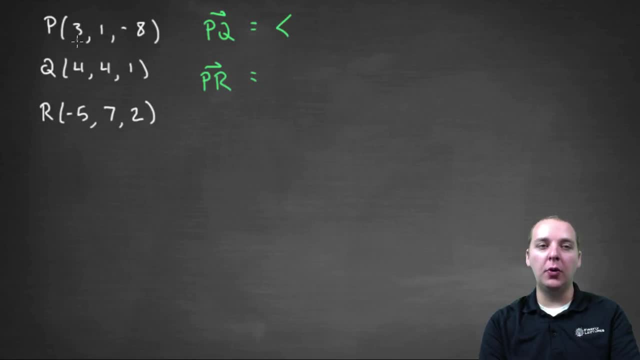 do this to put these in component form, we'll do terminal minus initial, as you probably recall. Uh, P, Q would be the vector one, three, nine. Now, where did that come from? I took four minus three, which is one, Four minus one, which is three. 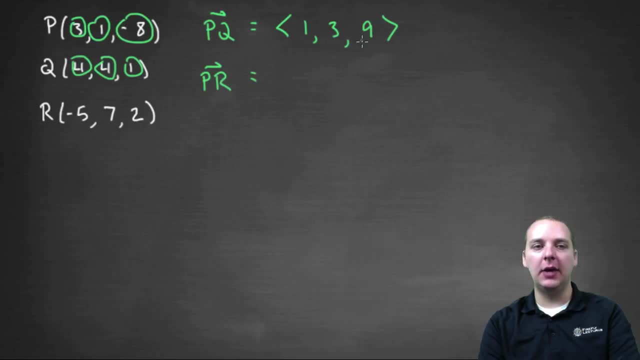 And one minus negative, eight which is positive, nine Terminal minus initial ending point, minus beginning point, Or at least the, the X, Y and Z values of those points. Alright, in the same way, let's see P, R, Uh, let's see here What is the vector from P to R. 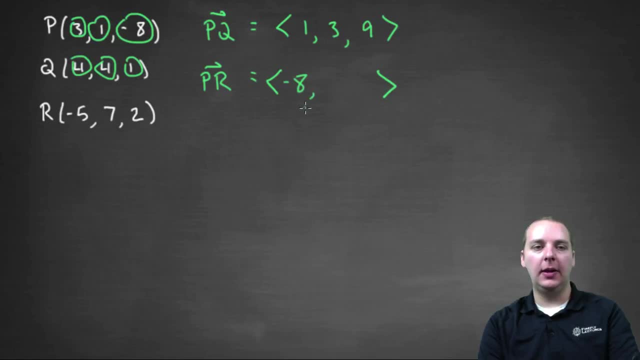 We have negative five minus three, that will be negative eight, Seven minus one, which is six, And two, minus negative eight, which is seven, And two minus negative eight, which is one, The 1,, 2,, 3,, 4,, 5,, 6,, 7,, 8,, 10.. And so on till we get the negative and the negative. 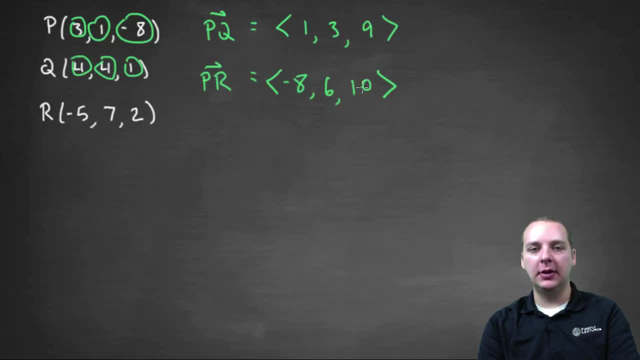 and the negative E: 1,, 0,, 0,, 4,, 5,, 6,, 7,, 6,, 7,, 8, and so on. Let's do that. Yeah, see, so eight, which will be positive ten. Alright, so now that I have these guys here, let's take 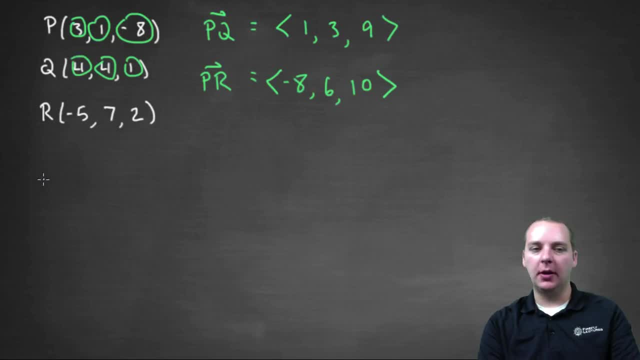 their cross product. hopefully you remember how to do that from previously in the course. So we'll take PQ crossed with PR, which we'll do that using a three by three determinate. We'll write IJK, one, three, nine, we'll write the vector PQ in the second row and then negative. 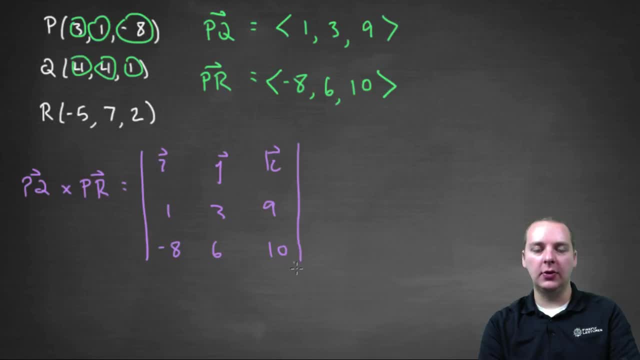 eight, six, ten, we'll write that vector in the third row. So this determinate will give us our cross product vector. Because it's not really the point of this particular video, I'm going to go through some of the algebra kind of quickly in computing this determinate. 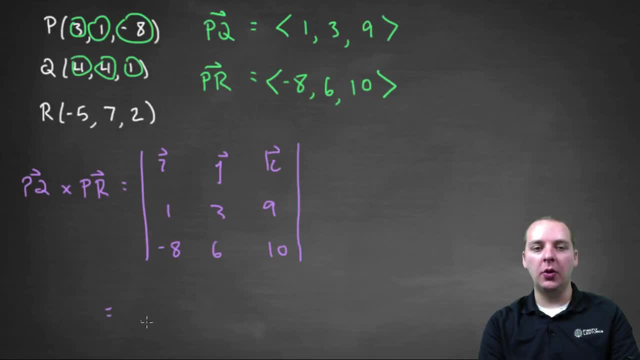 If you don't know how to do cross products, just go back and watch our video On cross products. let's see the I component will be, let's see, thirty minus fifty four. so that would be negative twenty four I, and then the J component will be ten plus seventy. 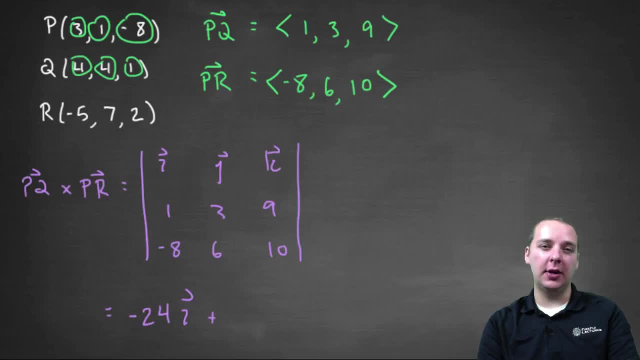 two, so we'll have eighty two J. actually, correction, it would be minus eighty two J Because the one times ten minus nine times negative eight is positive eighty two. but remember the overall signs when you're doing um, cofactor expansion or expansion by minors, the overall signs. you have a positive and a negative and a positive. so we're adding. 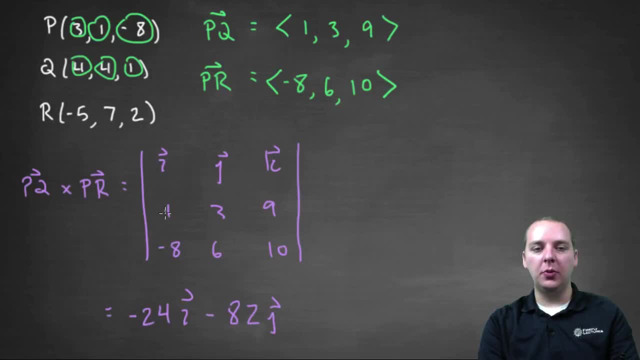 an extra negative here, and then the K component will be six plus twenty four minus negative twenty four, so twenty four and six makes thirty, so thirty K. So here's some crazy vector. now who is this guy? That's the guy that's going to be orthogonal to our two vectors, PQ and PR, which means as: 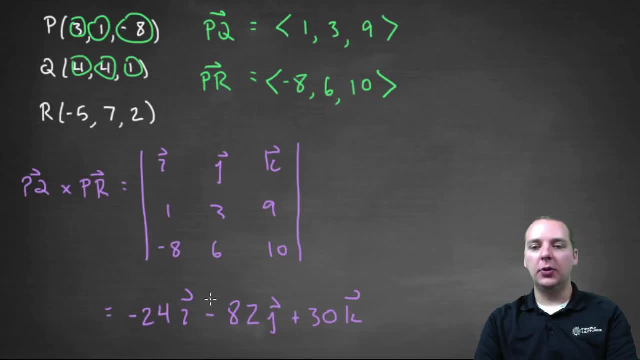 a result is also orthogonal to the plane. So in our equation, for our plane, this is going to be like your A, this is going to be like your B and this will be like your C. You can use any of these points- PQ or R, for all I care- in your, in your final answer. 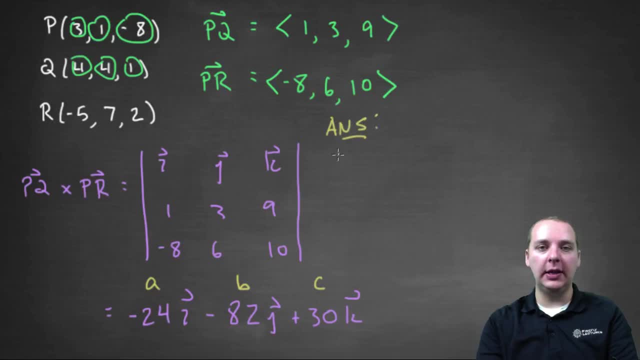 So here we go. final answer: the equation of the plane. you would have A times X minus X, naught. I'll just use point P, just because it's listed first, no particular reason. minus eighty, two parenthesis, Y minus one and then plus thirty times Z. plus eight equals zero.